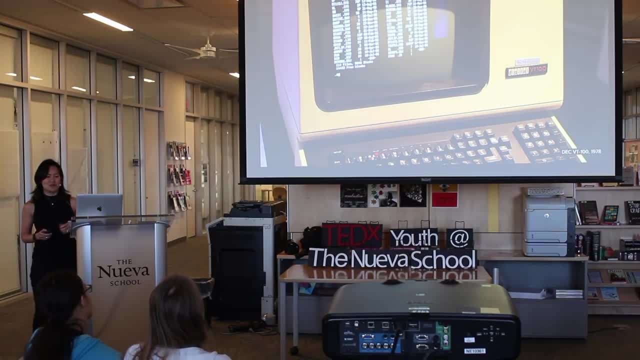 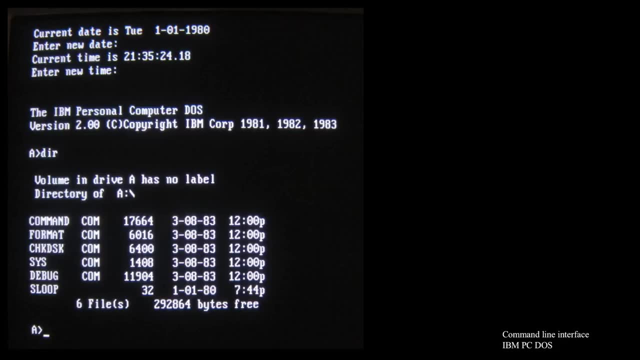 of interacting with computers, first on terminals like this, the DEC VT100, and later on personal computers, PCs, running UNIX or MS-DOS. The interface would consist of a command line shell, which would accept commands as text input and then convert the commands into corresponding. 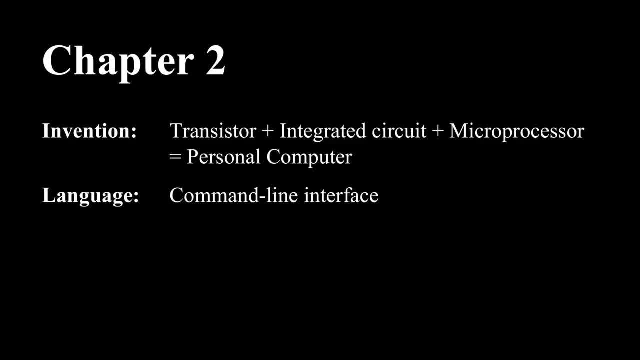 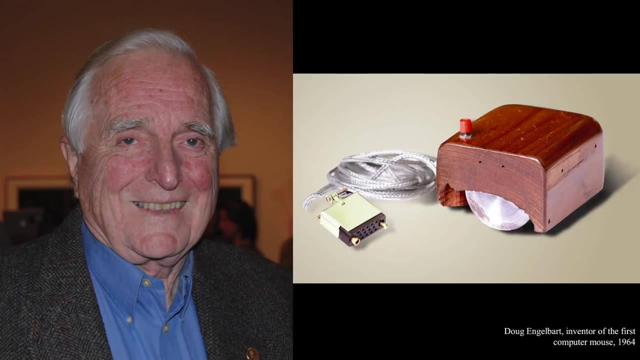 operating system functions. The advances made in computing technology, for example, were an opportunity for people to interact with computers in a different way. We moved away from physically manipulating bits to interacting with computers in a digital space on screen. The invention of the mouse by Doug Engelbart and the graphical user interface, or GUI. 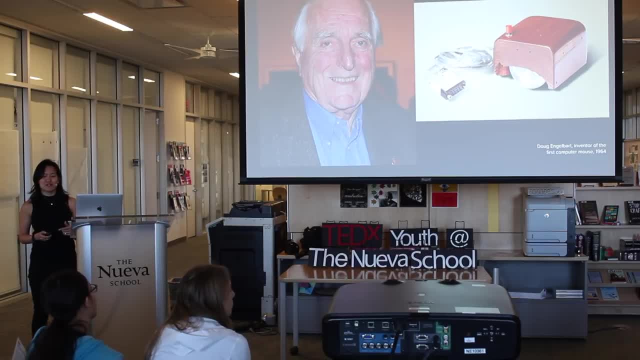 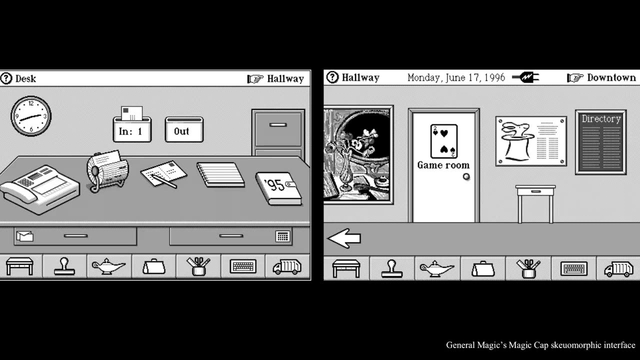 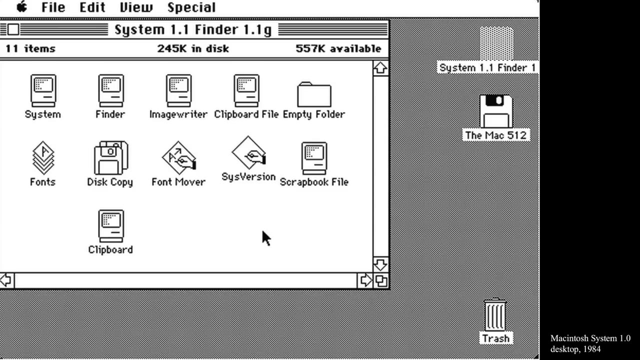 revolutionized HCI. It was really during this phase that the field was born, the field of HCI. Early attempts at graphical user interfaces were skeuomorphic and literally tried to create the physical world even in its most inefficient ways, The most successful style of interaction. 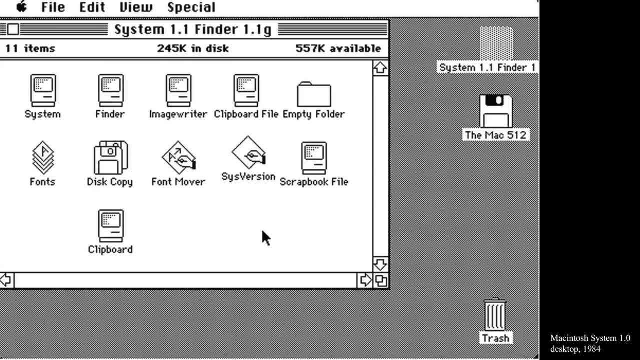 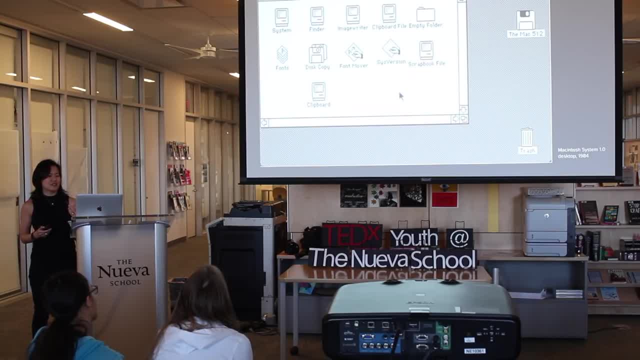 design has been what we refer to as WIMP, which stands for Windows, Icons, Menus and Pointer. WIMP interfaces are so ubiquitous that this is what comes to mind when we think of the term graphical user interface. although not all GUIs are WIMP systems. The language 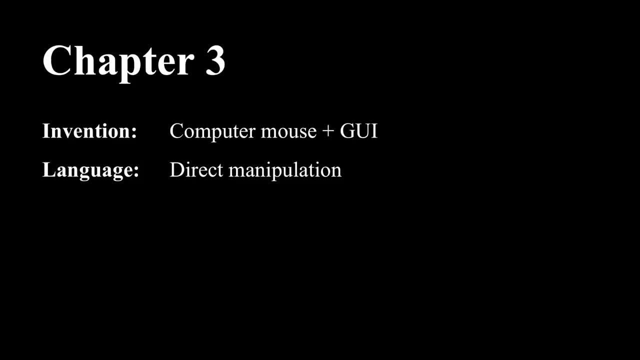 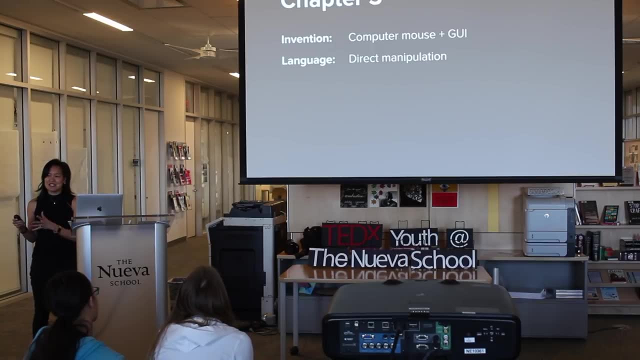 of HCI in a WIMP world is direct manipulation, complete with nouns represented by icons and verbs represented by menus or buttons, And with a GUI and a mouse. people could operate under a paradigm of: hey, you icon, go here into that folder or app. The Macintosh computer. 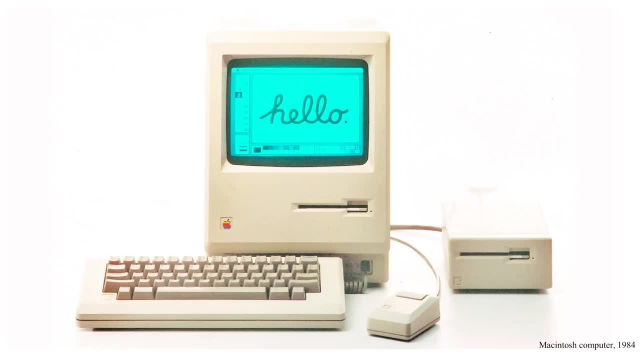 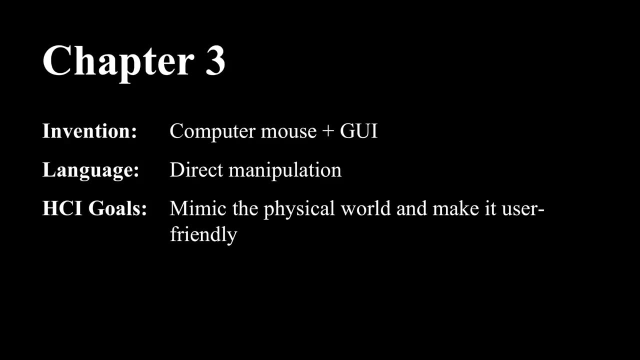 which exemplified the ideal GUI launched in 1984, with principles that emphasized directness, user control and real-world metaphor. The goal of HCI at this time was to leverage pre-existing paradigms of the physical world, without taking it too far, and make it user-friendly. 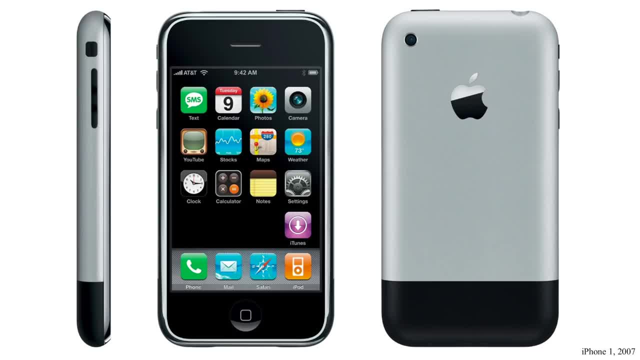 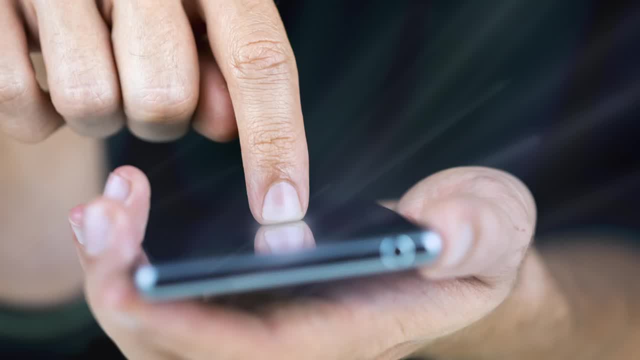 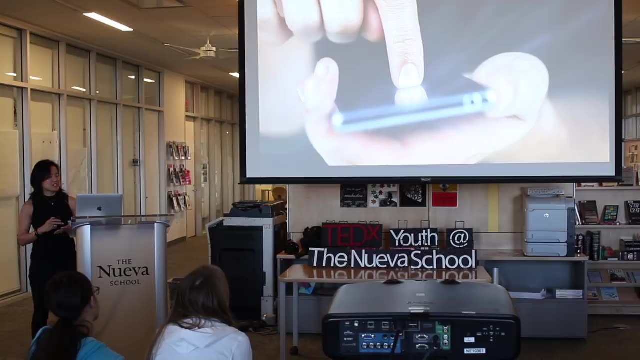 The birth of the iPhone and Android-based smartphones put the power of computing in everyone's pocket. By using our fingers instead of a mouse, direct manipulation is even more direct than a WIMP interface. We swipe to scroll. we literally drag objects by dragging. 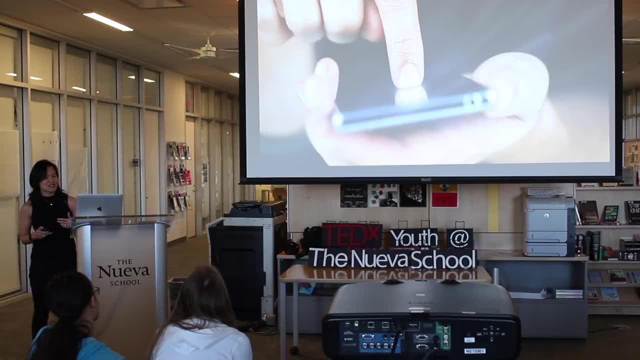 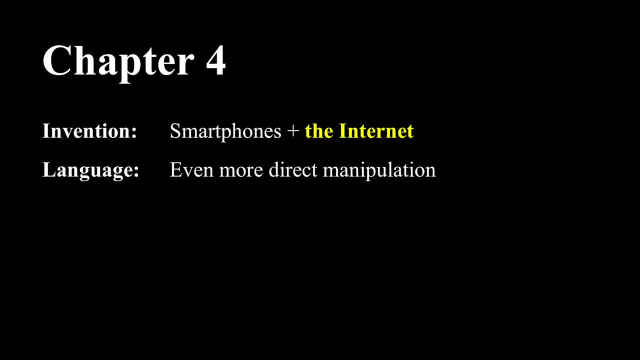 our fingers. It's still direct manipulation, but the language has evolved to meet the form and the capabilities of the computing device. Now, early handheld computing devices were introduced before we had new technologies. The first time we had new technologies was the ubiquitous broadband, So functionality at that time was typically limited to personal. 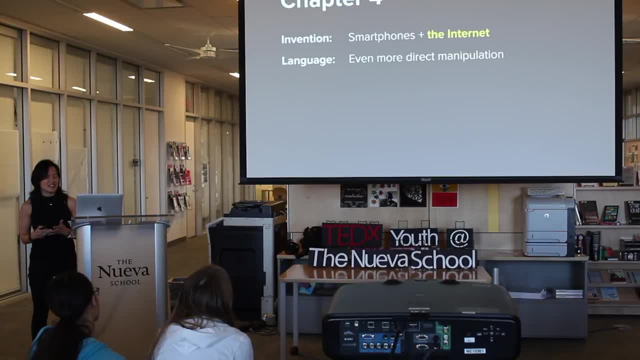 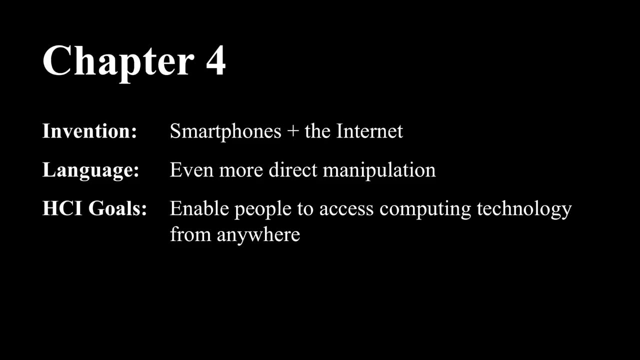 digital assistant features like calendaring, note-taking, contacts management And the internet is what really enabled smartphones to take off and be not just useful but extremely addictive, And with the power of what once used to be a supercomputer now in the palm. 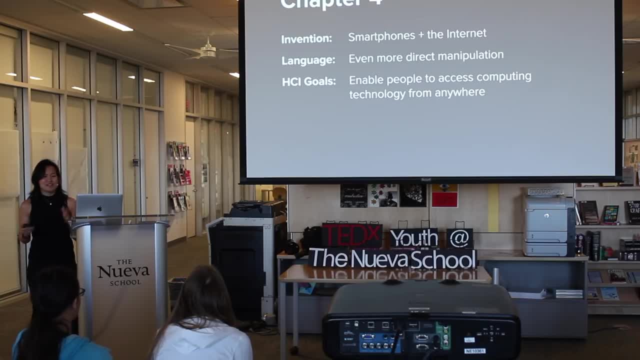 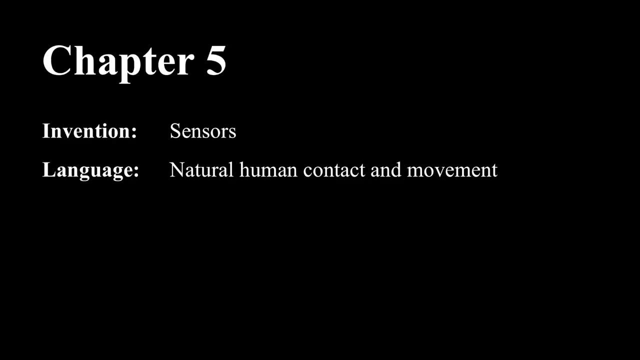 of your hand. we enable people to access computing technology from anywhere Now, whereas in the first phase of computing we were bringing the physical world into a digital space. sensors enable us to use natural movement to bring a digital world into a physical space. The Xbox Kinect made playing video games a physical endeavor. The Fitbit digitized. 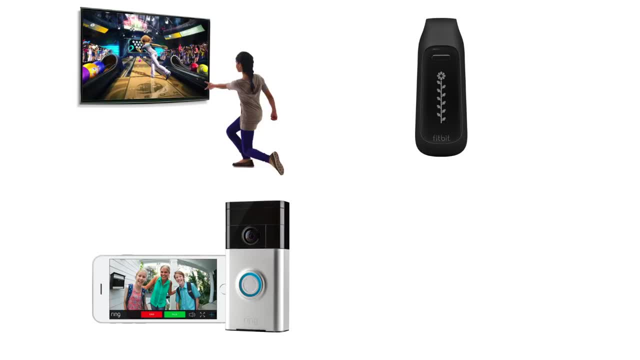 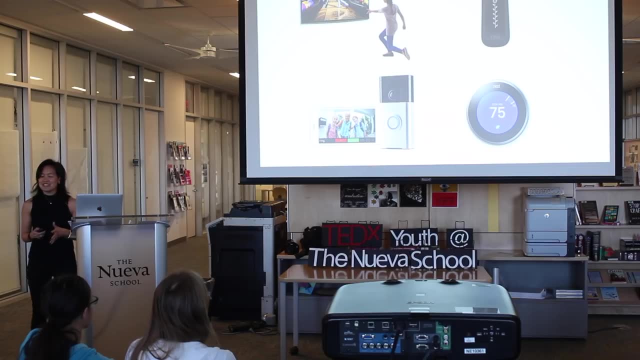 our physical activity Ring allows us to talk to visitors at our door even when we're not at home, And Nest made our thermostats smarter by adapting to our usage patterns in the home. I'd like to highlight a few more companies that are doing interesting work in this area. 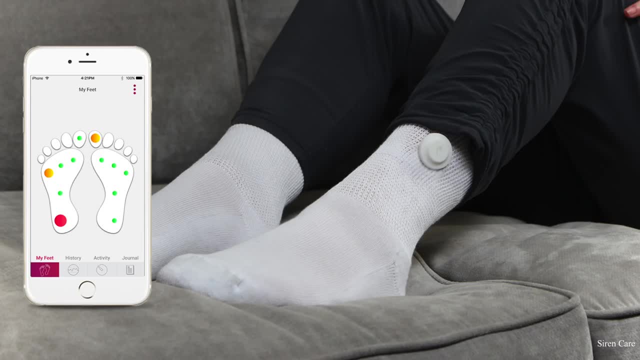 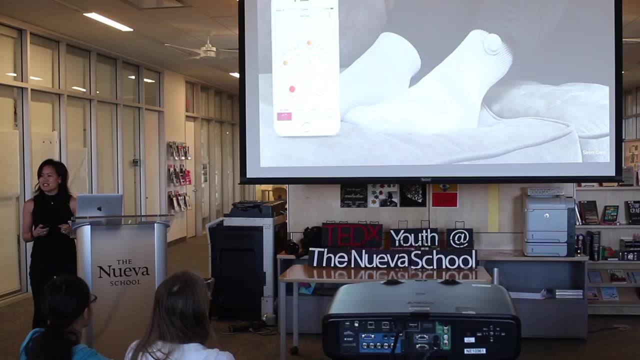 particularly in health tech. Iron Care has created smart socks that use temperature sensors to detect inflammation in real time for diabetics. Diabetes patients are prone to foot swelling and that can lead to infection or amputation if the foot isn't checked. Conductive thread is woven into the 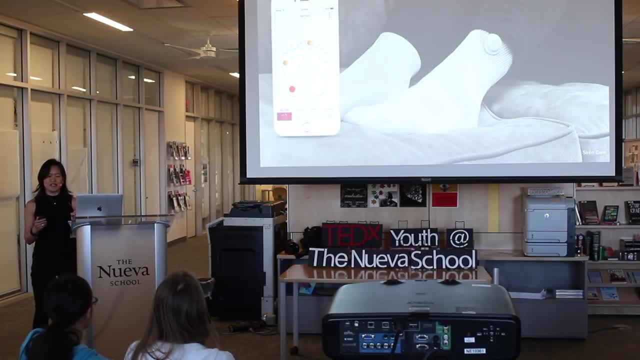 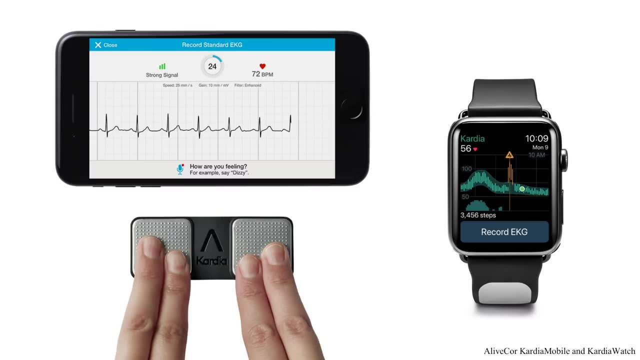 fabric of the sock to detect where there's inflammation, and all this information is uploaded to an app on your smartphone to alert you to an issue. Here's another company, AliveCore. They offer a mobile FPC device that can be used to detect inflammation in real time. 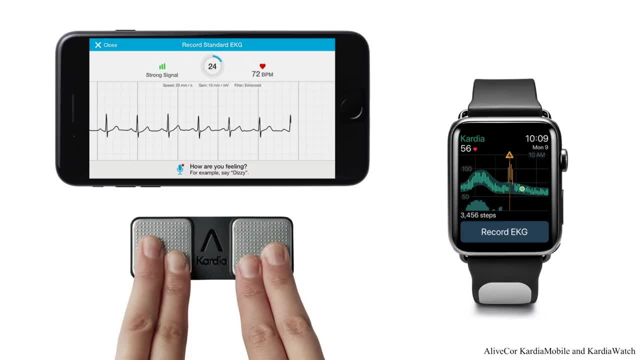 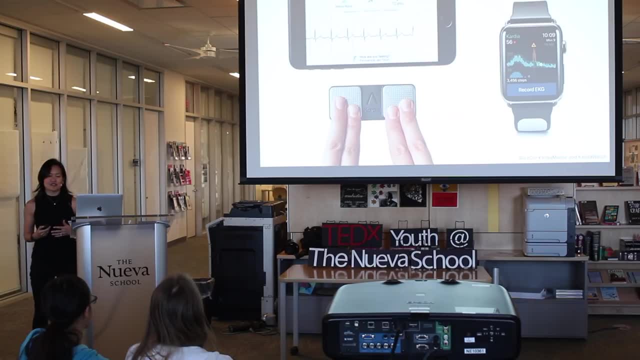 AliveCore is an FDA-cleared EKG monitor targeted towards patients who have atrial fibrillation. AFib patients have an irregular and often rapid heart rate that can increase their risk of stroke, heart failure or other heart-related complications. AliveCore offers two ways for 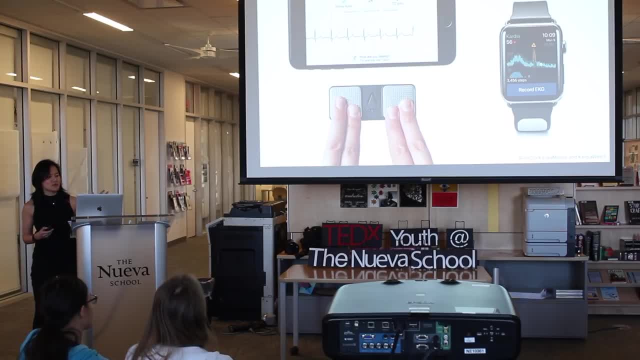 people to monitor their heart: CardiaMobile, which is an attachment to your phone, and CardiaWatch, which is a replacement wristband for your Apple Watch. A notification is sent to the user to record an EKG if the heart rate is too high. If the heart rate is too high. 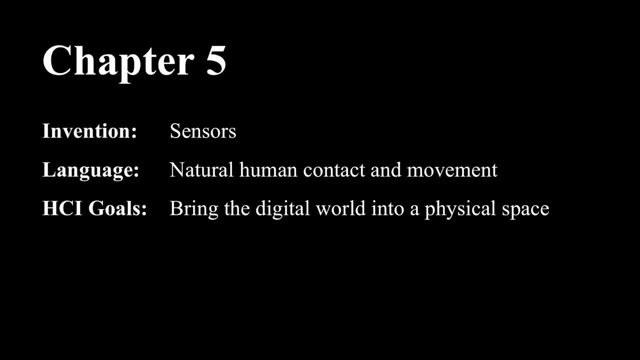 the user's heart rate appears inconsistent with the user's activity level. Now, theoretically, it could go further. All the data is stored in the cloud and AliveCore could mine all of the data to make predictions based on what they see. For example, if your 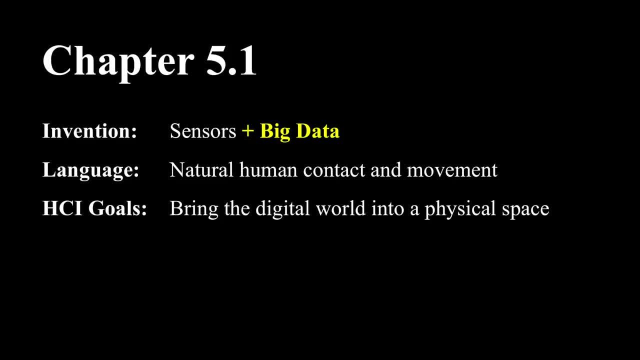 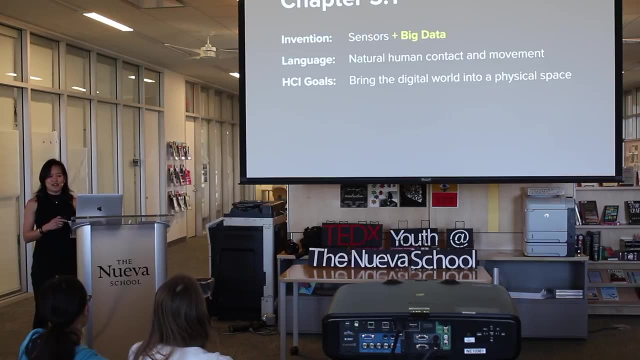 EKG reading mimics the patterns in other patients hours before they had a heart attack. AliveCore could send you an alert and advise you to take necessary precautions to avoid an imminent heart attack. So as computing moves beyond devices with screens, the language of HCI similarly evolves. 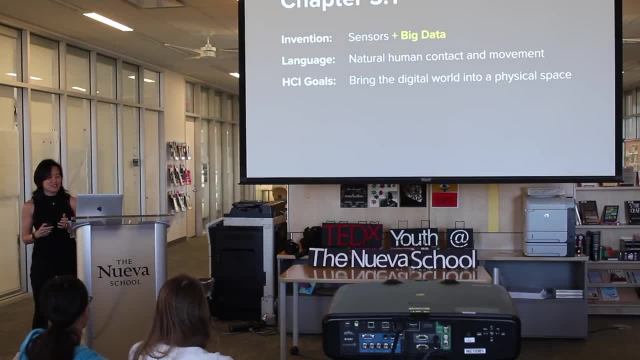 How do you design without a screen? As we bring the digital world into a physical space, how do we deal with the ethical and privacy issues surrounding constant instrumentation and mass collection of personal data? I wrote this talk before all the news came out of Cambridge Analytica. I think it's particularly 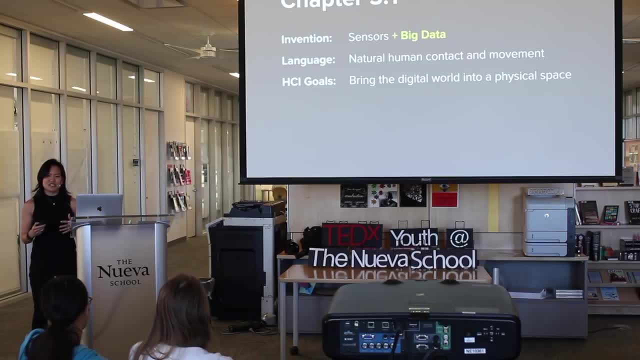 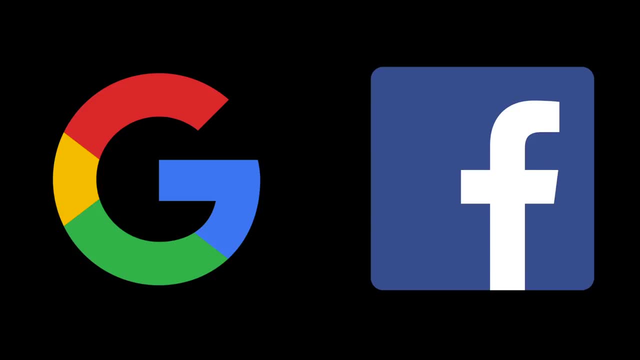 timely and relevant. As sensors become ubiquitous, we increasingly track every aspect of our lives. We reach a point where computers know more about us than we know about ourselves. So already Google and Facebook algorithms know exactly how you feel and countless other things that you may not even know. Facebook only needs 10 likes from you to outperform. 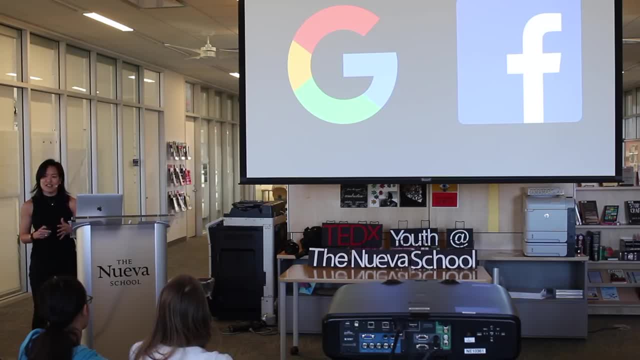 predictions from work colleagues about your preferences, personality and dispositions. They need only about 70 likes to outperform your friends, 150 likes to outperform family members and 300 likes to outperform spouses. So if you have clicked 300 likes from your Facebook account, Facebook can predict your. 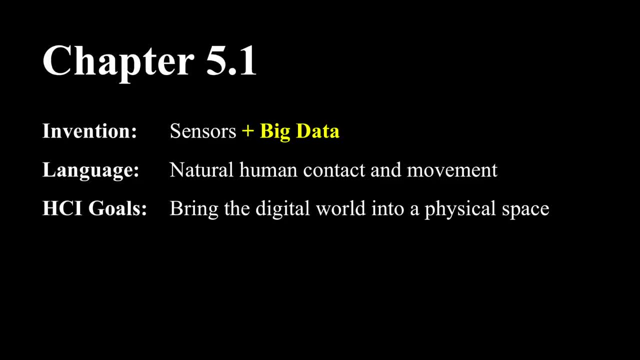 opinions and desires better than your own life partner. Now imagine if Google or Facebook read every single email text message post we ever wrote, every photo we ever took, and combined that with knowledge of our heart rate, blood pressure, hormone levels in real time as we move through everyday life. They would be better equipped. 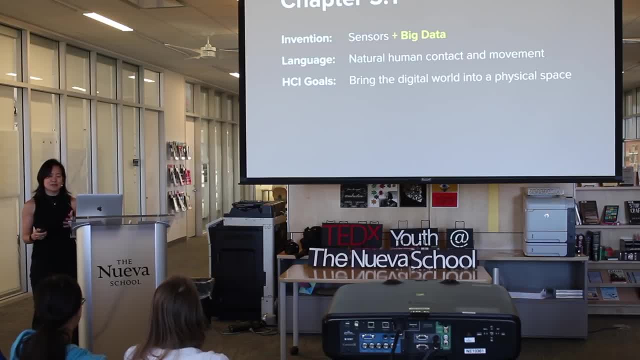 to tell us how to vote, mate, to choose how to spend our time far beyond what we are consciously aware. In the same way that we rely less on our sensory direction and navigation, now that we have GPS, you may decide to stop listening to your feelings and start listening to these external. 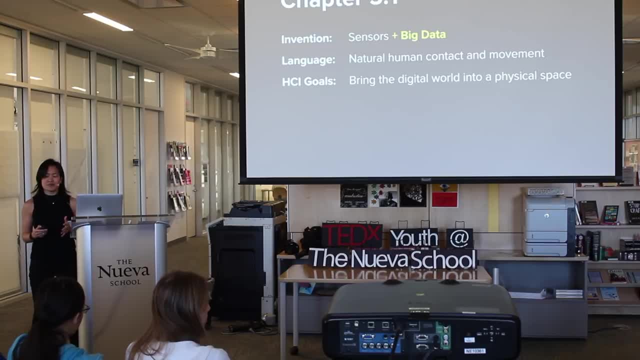 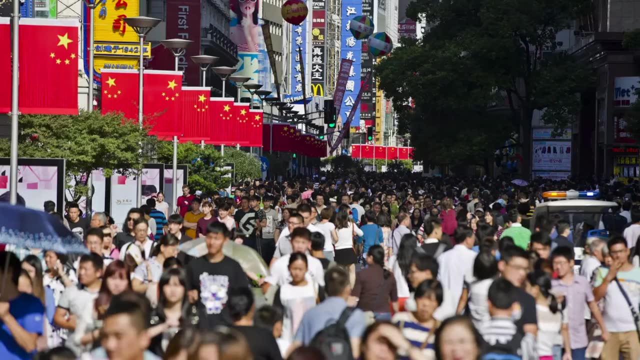 algorithms instead. This could lead to a scenario where algorithms would be better equipped to vote on your behalf, obviating the need for democratic elections. In China, the government is testing a new way of social control that ranks citizens based on their social and financial 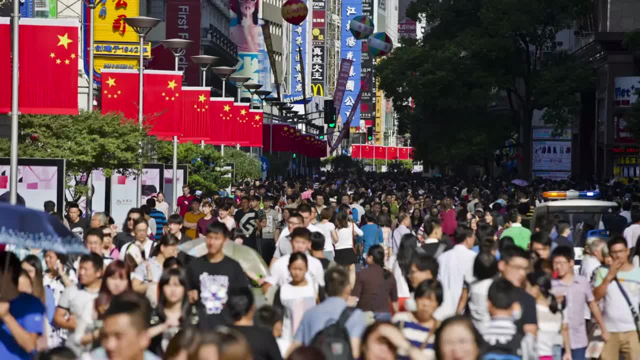 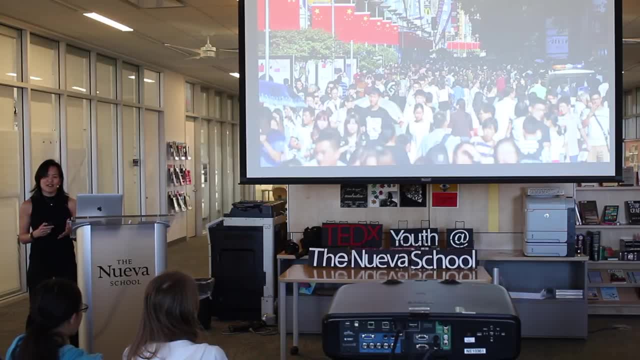 behavior. The social credit system would use facial recognition to evaluate individuals' day-to-day behavior and generate a credit score for each person. So minor violations like jaywalking or jumping the transit ticket line could decrease one's social credit in the system, thereby affecting their ability to get a loan or travel abroad Now strict. 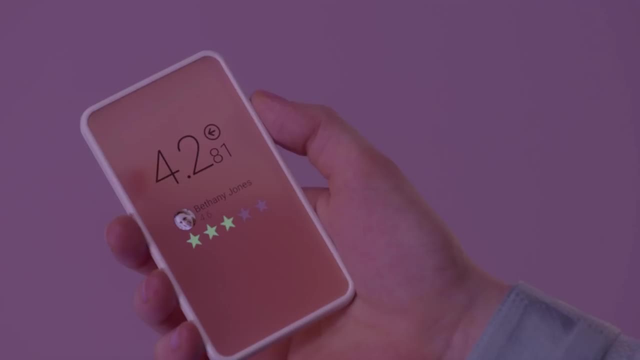 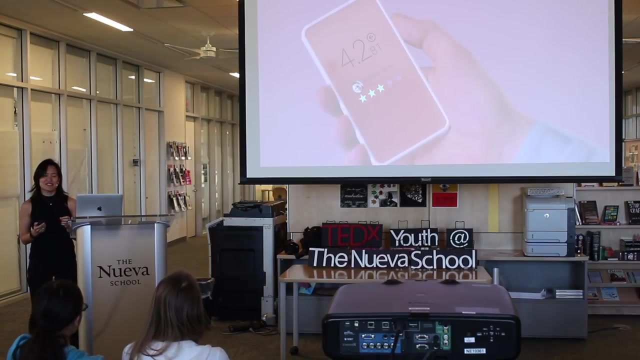 privacy laws in the US may protect us, But they can hinder us from making the best prediction when it comes to our health care decisions. while dealing with a genetic database, Since this is all based on statistics, the size of the company's database is key to making accurate predictions. Chinese disregard for 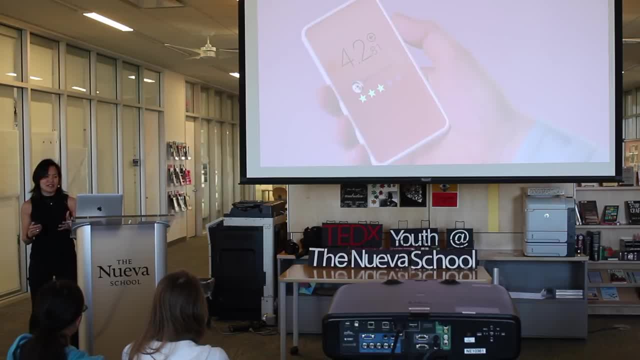 privacy may give them an advantage in the area of health and medicine. That, and the relation between security and privacy, is a major issue. So in 2011,, after the end of the crisis, China began to close its borders on its own economic security plans and grow in size and industry with a new disruptive policy. 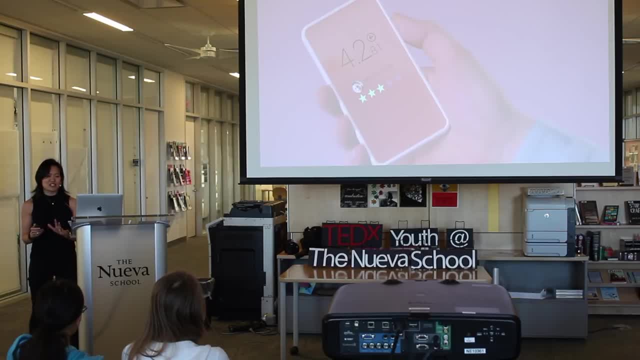 And this was the first time the country has owned a private bank. So that's why I really appreciate the top six of the data set by the pandemic. We have a lot of data coming in. We're looking at all of this. We're looking at the stock market. We got to look at this. 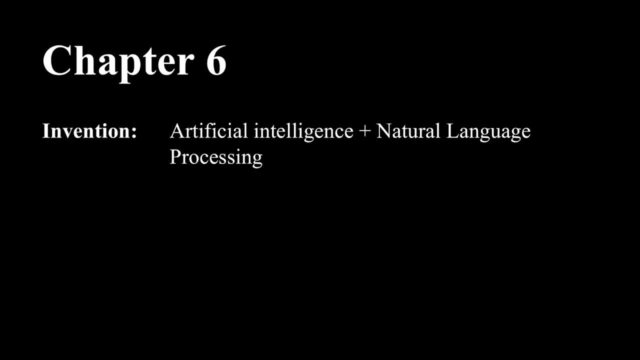 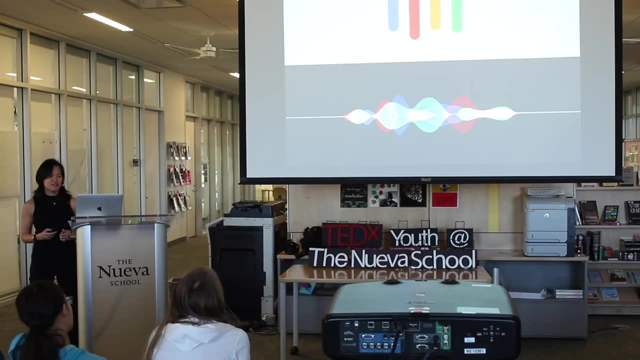 But many, many years ago, there were only three or four companies that were able to and medicine over the US. So in 2011,, Apple rolled out Siri. Google now launched in 2012,, marking the beginning of a new phase. 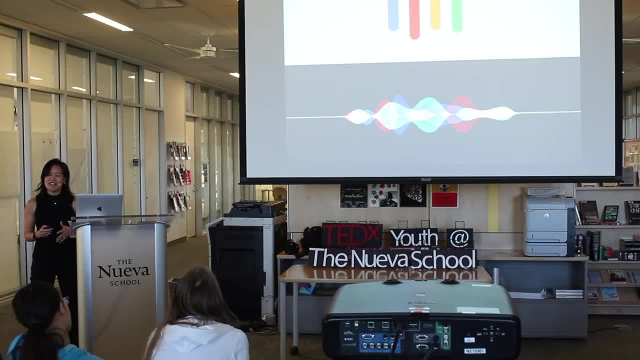 where apps use natural language to answer people's questions. We now have fast enough computers and data where we can actually train large neural networks, and as we train them with more and more data, the performance improves accordingly. In 2015,, a 31-year-old man named Roman Mazarenko died while crossing the street in Moscow. His death was a devastating loss for his best friend, Genia Kuda. At the time, Kuda had been building a messenger bot that could do things like make restaurant reservations, And she fed her text messages with Mazarenko. 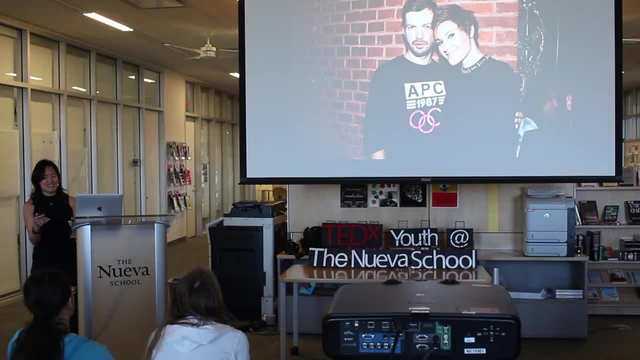 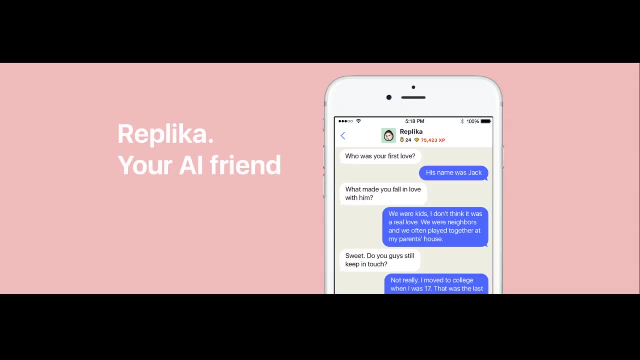 into her neural network and created a bot in his likeness And as a memorial to Mazarenko. Kuda replicated his personality and could talk to him again via a chatbot, And so thus Replika was born. The chatbot uses a deep learning model. 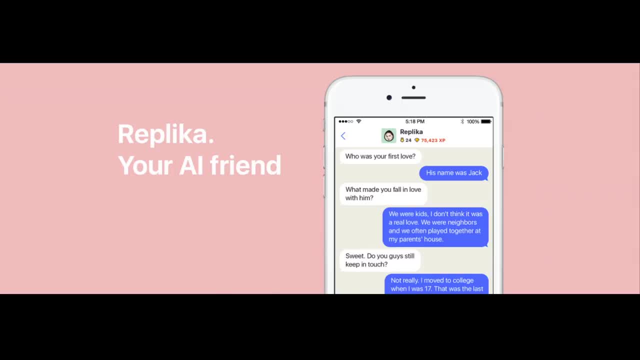 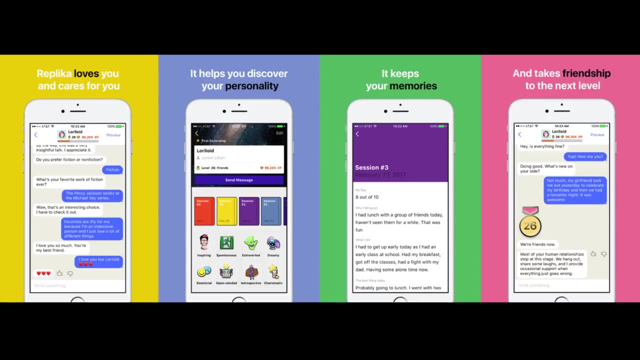 which learns how to mimic how humans speak in order to simulate conversations. The version of Replika that exists today is used by people who seek emotional support. It's not a substitute for Siri or Alexa or Google Assistant. People are using Replika to talk about their feelings. 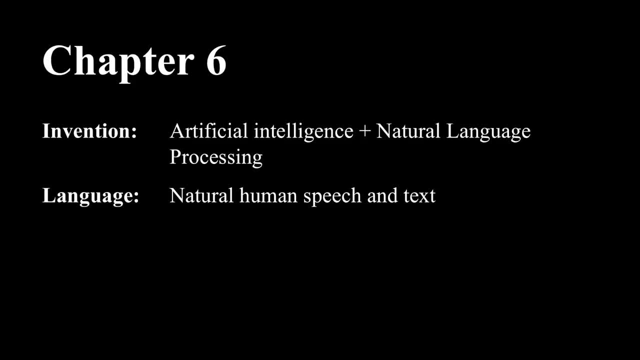 AI researchers and roboticists are testing the limits of how much machines can learn to mimic and respond to human emotion. These are the big questions the world of HCI seeks to answer now. How do you get a machine to think and act like a human? 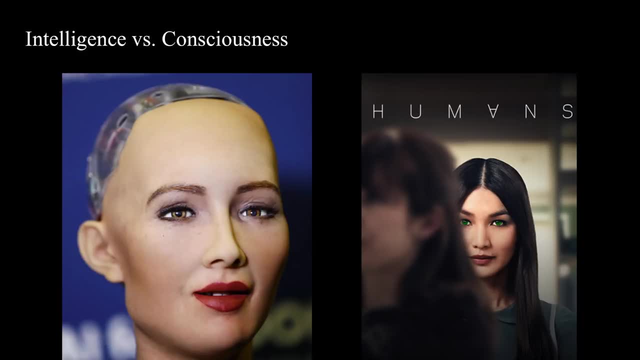 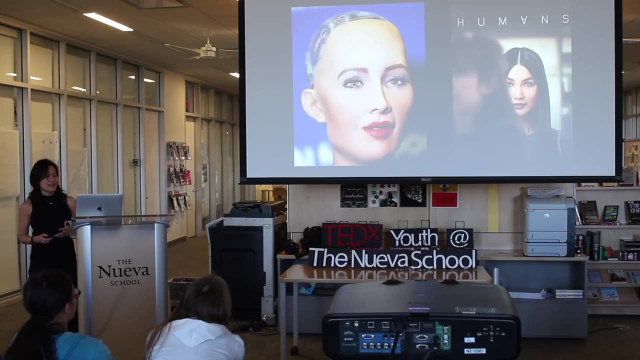 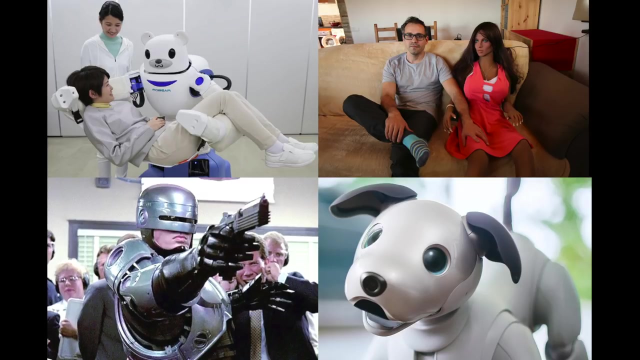 What does it mean to be human? Are organisms just algorithms? And is life really just about data processing? Is consciousness valuable? And what about love or human connection? What kinds of relationships do we want to have with machines? Are they our friend, assistant, sentient being law enforcer, pleasure partner? 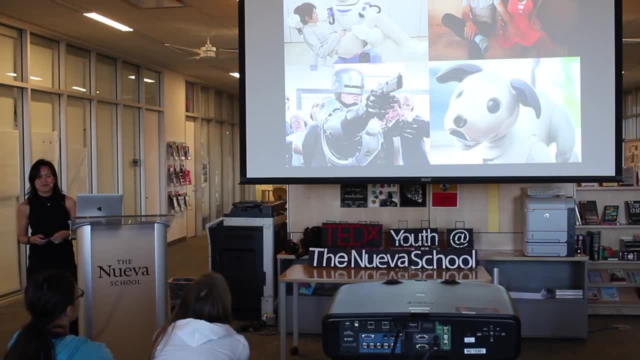 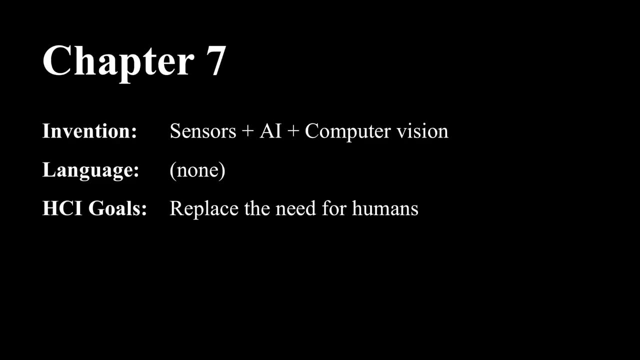 What is the role of the machine and what is the role of the human? As machines are increasingly trained to think and act like humans, their abilities surpass ours, And many of the startups that I work with are using human users to train the machine learning algorithms. 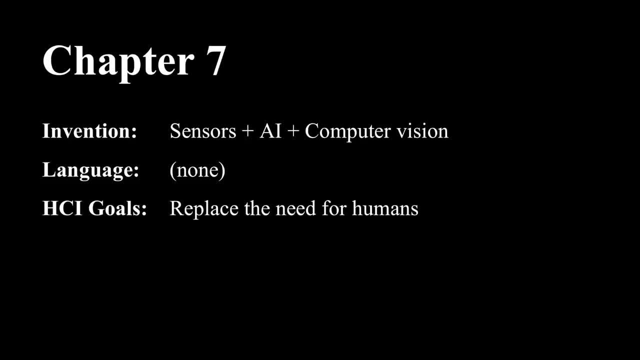 so that machines can do the same work at a much faster, much larger scale. And as this becomes realized, as the technology becomes realized, the goal of HCI is no longer a goal unto itself, but a goal to be removed. In fact, one of the executives 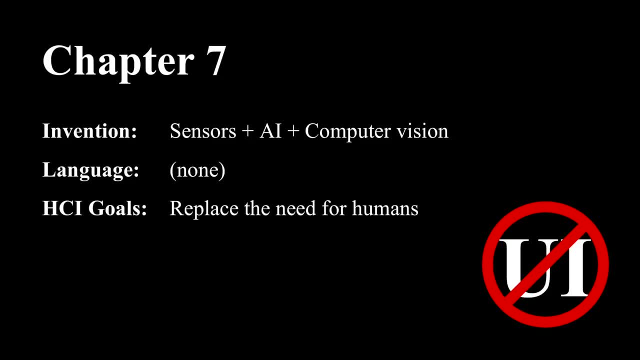 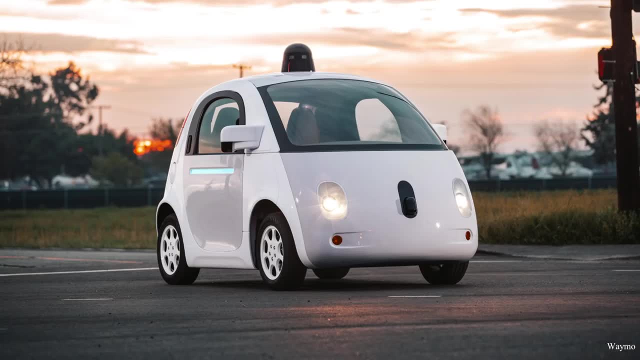 that I worked with boldly proposed a quarterly no UI goal where the goal would be to launch at least one feature per quarter that requires no human user. But what happens when there's so much automation that humans have no role in decision making when their lives are at stake? 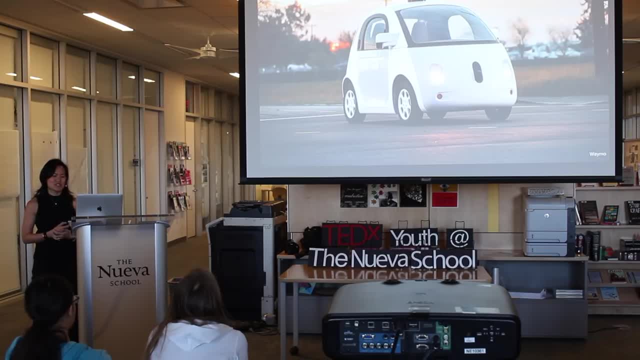 And we've all heard about the Waymo- sorry- the Uber accident that happened earlier this week. Imagine you're riding in a self-driving car and, because there's still some cars on the road that are not autonomous, there's a scenario where your car could collide with another. 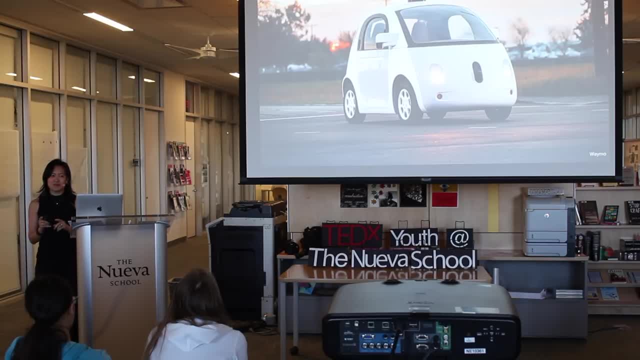 because it's not coordinating with the car. Now should your vehicle be programmed to save the passenger's life, which is you? Or what if the car is about to hit a busload of people and there are many more lives at stake? Or what if that busload of people is filled with children? 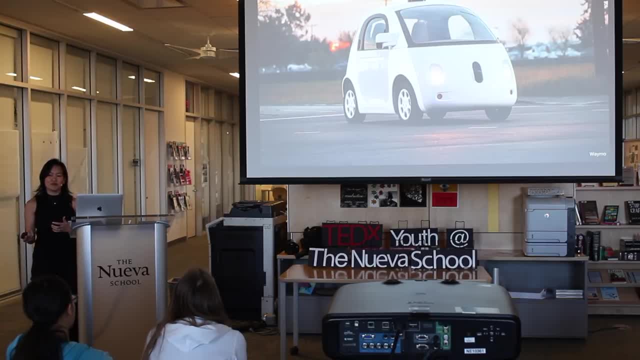 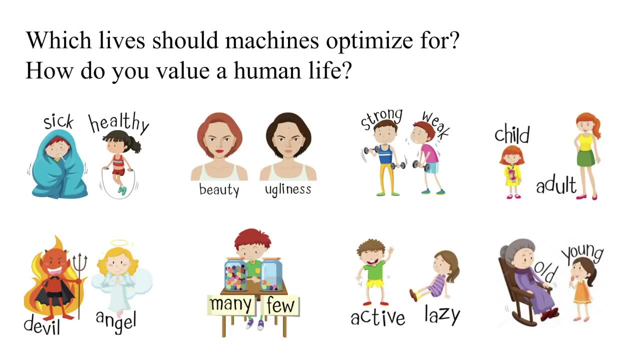 What if the other victim is wealthier than you or younger than you or healthier than you? Which lives should our machines optimize for, and how do you value a life? Machine values reflect human values, and a human-centered approach to AI means that our machines 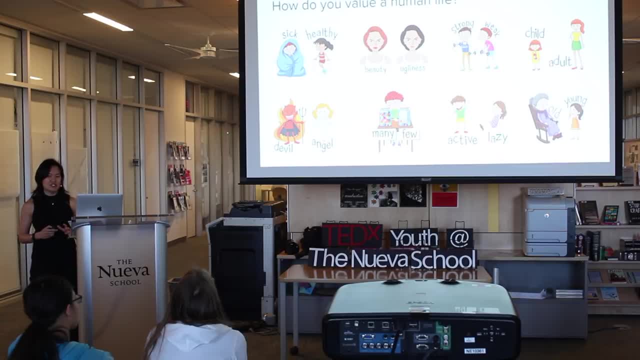 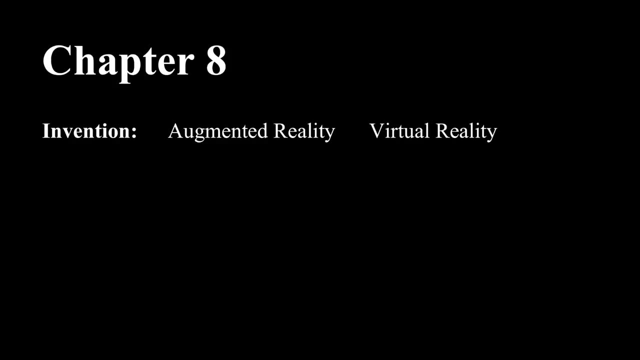 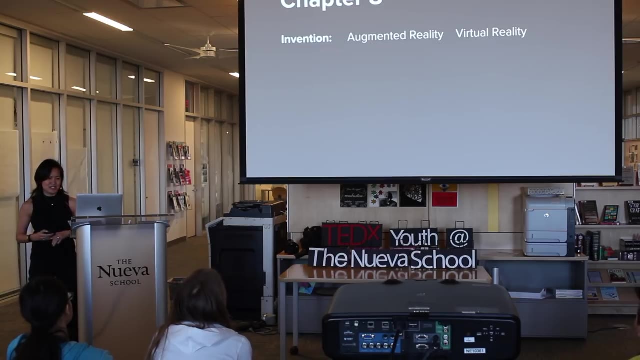 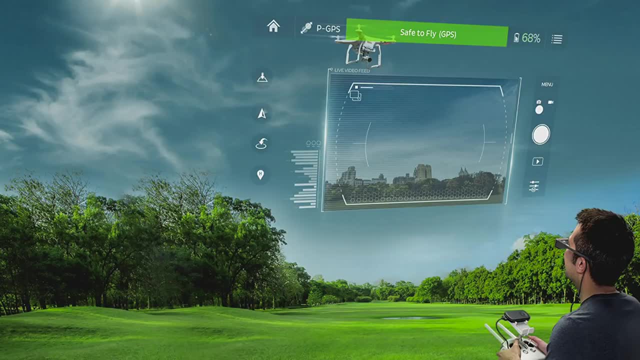 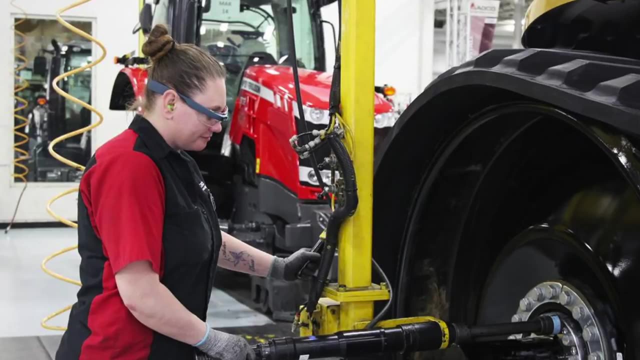 So I'm going to talk about AI in a little bit, For specialized applications like flying a drone, or for business use, such as on factory floors or in the operating room. But there's an increasing consensus that augmented reality will be the new platform in computing. 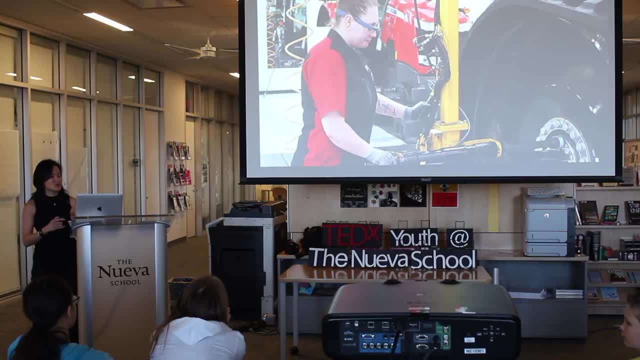 In these contexts of use. the goal of HDI is to connect the physical world with the virtual world. For example, how might data on demand overlaid with the physical world help people do their jobs more effectively or efficiently? How might these systems be designed? 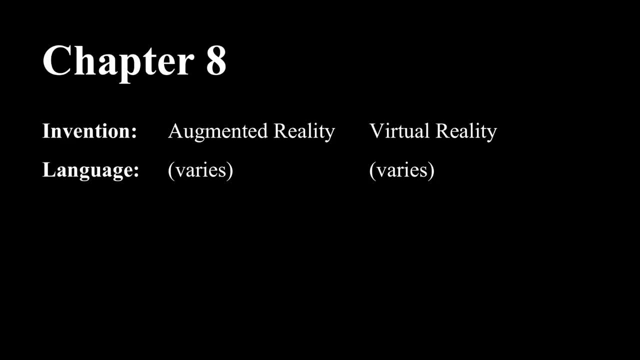 so that they can be used in the real world and not be used in a hands-free environment. Now, the software for AR and VR systems continue to evolve, and thus the language for interacting with them continues to evolve and vary, But they all leverage natural human movement mediated. 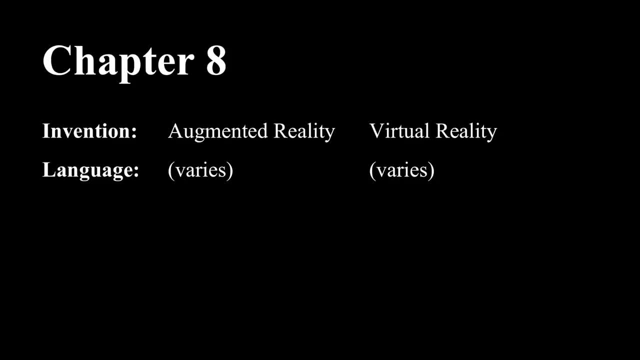 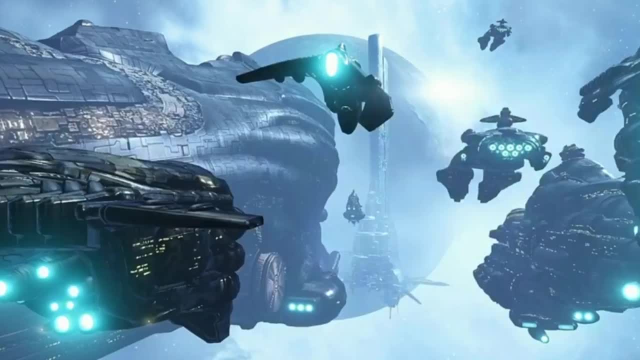 by some kind of display, whether it's your retina or screen or sensors. Now, whereas AR aims to connect the physical world with the virtual world, VR aims to bring humans into the virtual world. Virtual reality stands to occupy people's time and attention. 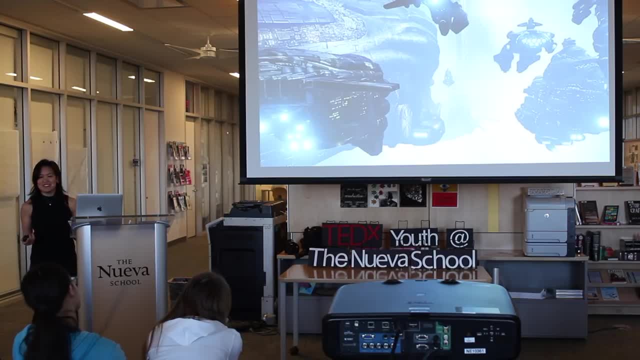 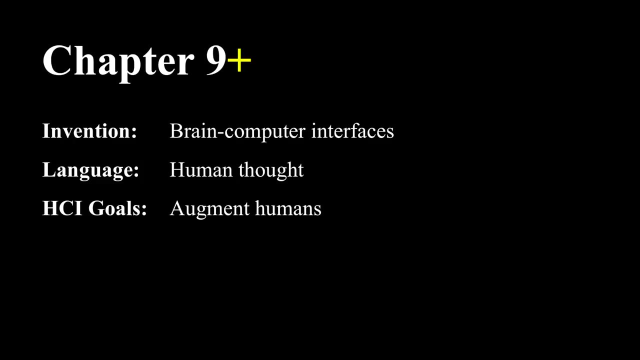 either as entertainment or as an escape from reality, or both. And in a world where robots have taken over most jobs, virtual worlds may be the place where people seek a sense of meaning and purpose for their lives. Now, no other invention has the potential. 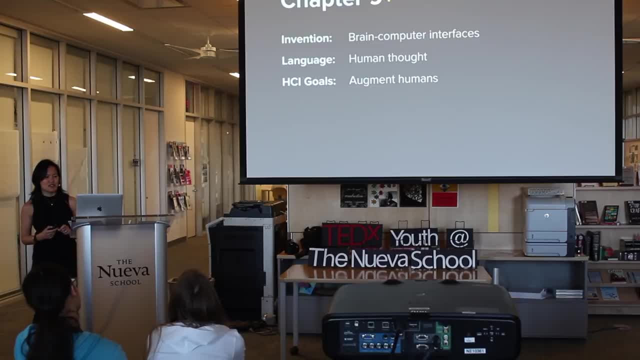 to radically change human-computer interaction than brain-computer interfaces. Now, today, all the interaction with a machine or computer is done through a device between you and the technology, whether that's a mouse, a keyboard, a computer, a computer. 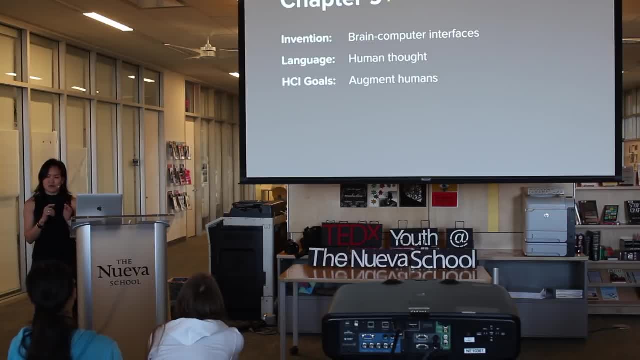 a keyboard, a joystick, a screen or a sensor. By removing that device and directly decoding the signals from our brains to the devices, we break through to a whole new kind of interaction between humans and machines. There's one company called Control Labs. 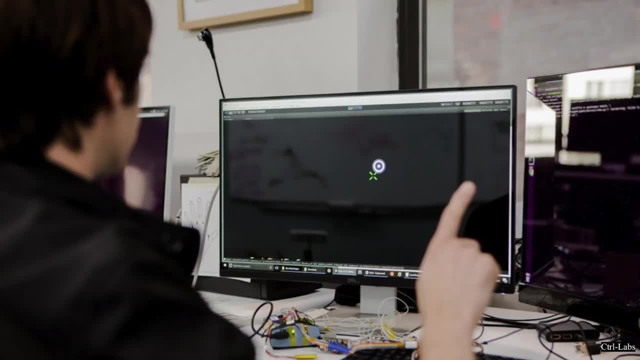 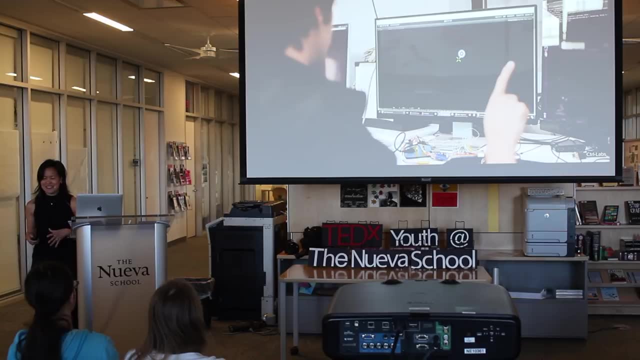 that is doing just that. The first thing that they want to fix is the experience of texting on phones. Imagine not needing a keyboard to enter text into a mobile device. What if we could send a message to our loved ones from our pockets, with our hands still in our pockets? 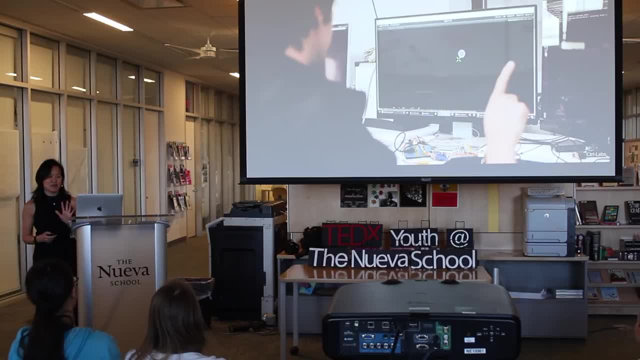 There's literally no interaction with a machine today, neither with the phone or the computer or any kind of robot, that this technology doesn't ultimately turn upside down. We often engage in research around human augmentation with the noble goal of curing disease or helping the disabled. 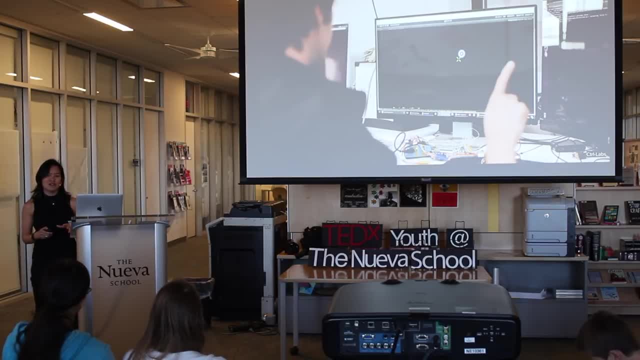 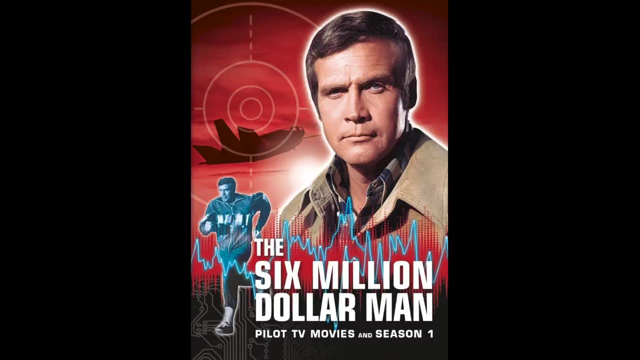 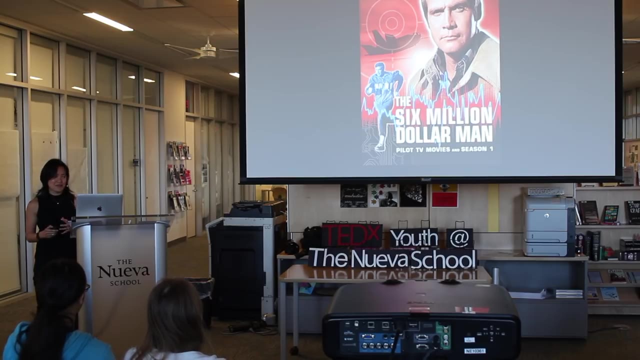 But inevitably groundbreaking inventions are often used to upgrade normal healthy humans as well. Imagine future: humans may enjoy upgraded physical and mental abilities that will enable us to hold our own against the most sophisticated non-conscious algorithms With the help of genetic engineering, nanotechnology. 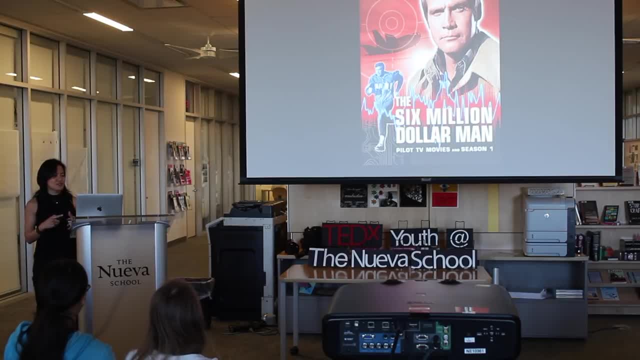 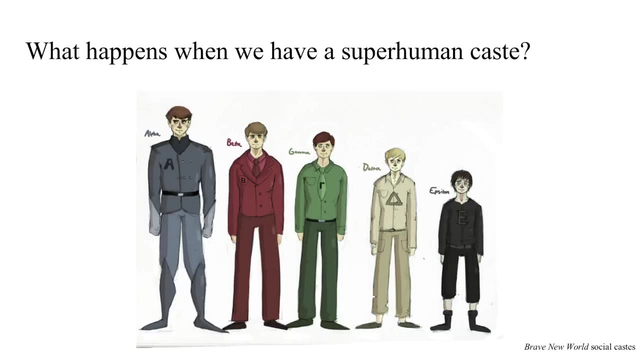 and brain-computer interfaces, we may reach a variant of superhumans made available only to a select few, namely those who are wealthy enough, who can afford it, And this could result in the creation of a new superhuman system. What then becomes of our society when we have a cast of people? 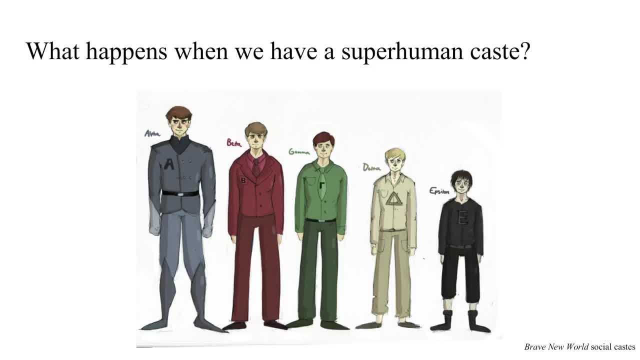 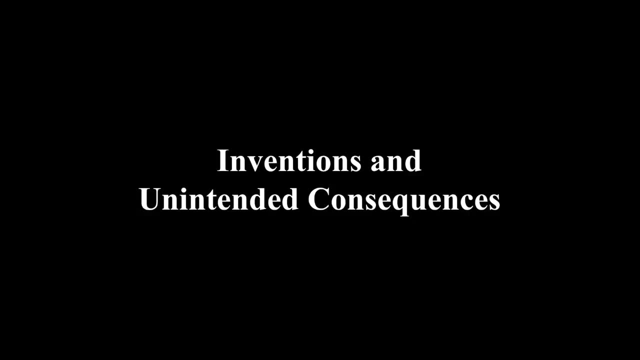 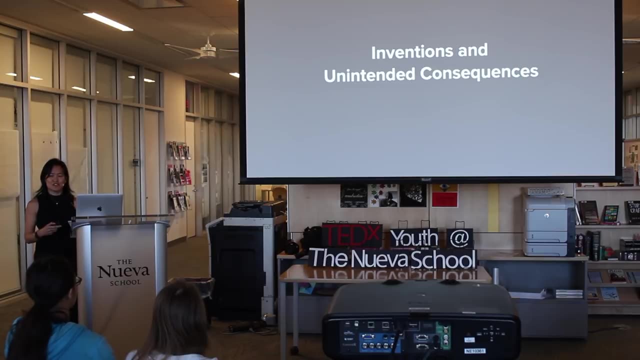 who are engineered to be superior to normal humans. How will that change the way we perceive and value human life? Now, in the early days of human-computer interaction, students like myself studied human cognition and perception, which allowed us to make technology useful and usable. 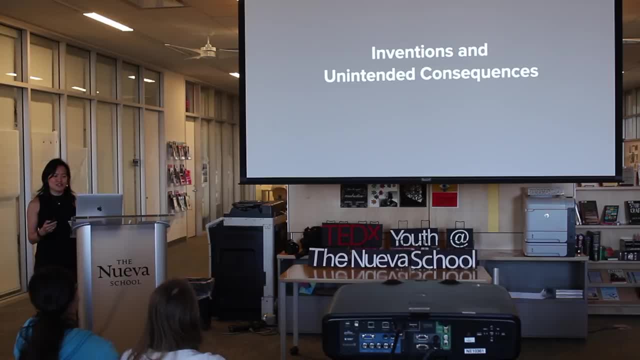 We could not have imagined that a service for sharing videos would be used to radicalize people, or that the very social media platforms used to move the Middle East towards democracy would be used to disrupt the US democratic process in the 2016 election.